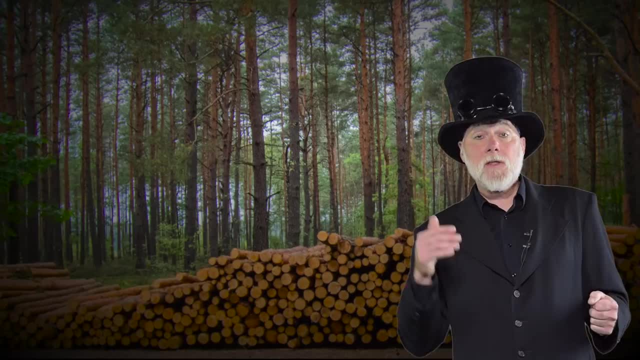 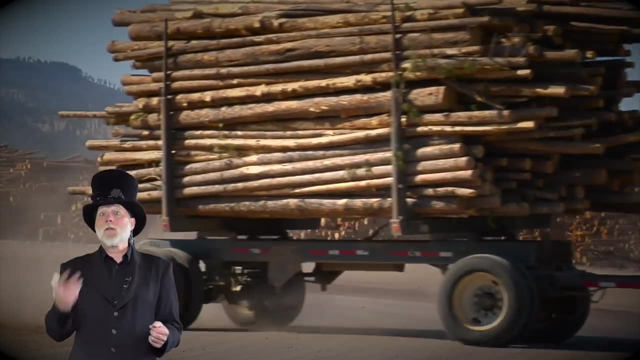 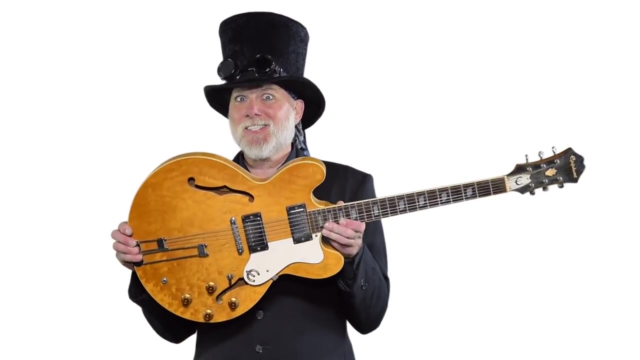 Trees are renewable. They can be used by humans and then replenished by nature in a relatively short amount of time. Here's how it works: We can cut trees down for lumber, to build houses or furniture, or even use the wood to make something like this awesome guitar. 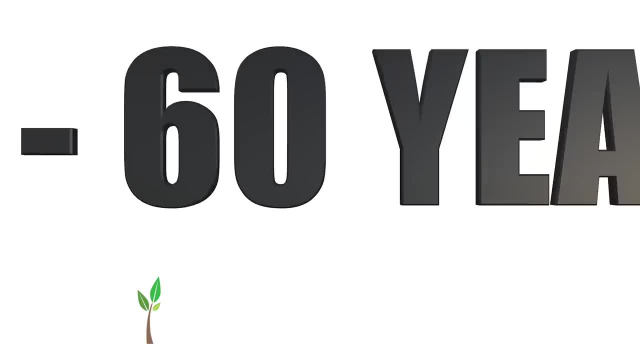 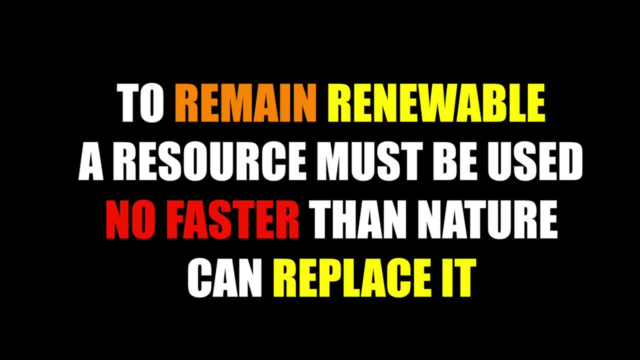 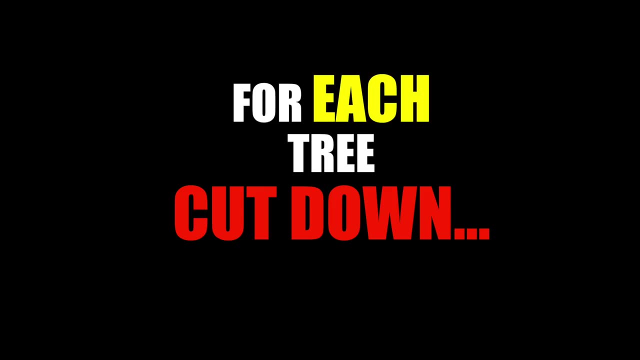 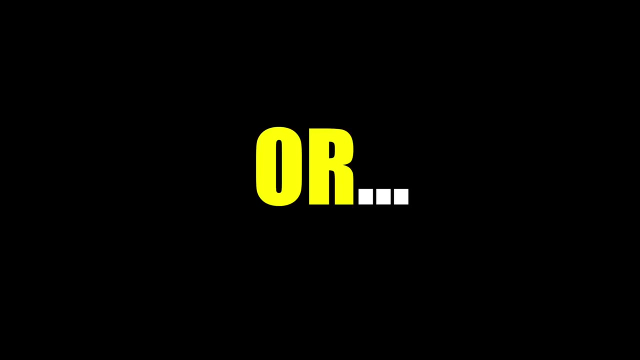 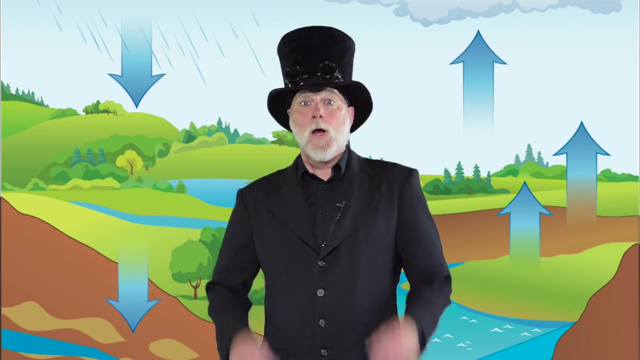 In place of the tree we cut down, we plant a seedling And in 40 to 60 years there's a full-grown tree to take its place. Water through the water cycle is replenished or renewed much, much more quickly. 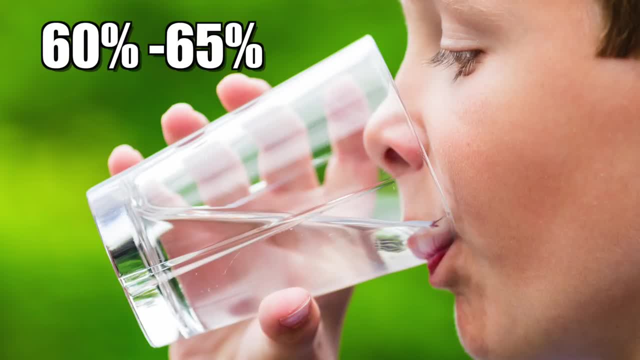 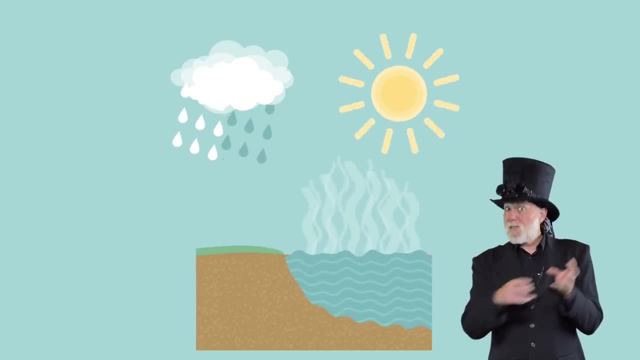 The water that we drink- which, incidentally, makes up most of our bodies- is replaced in a short period of time by the water cycle: Evaporation, condensation, precipitation, See, Replenished by nature. That's what makes it renewable. 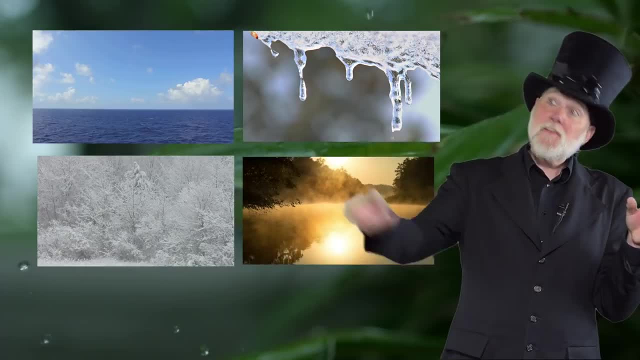 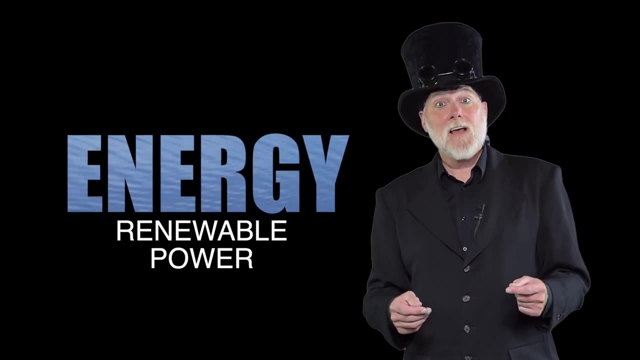 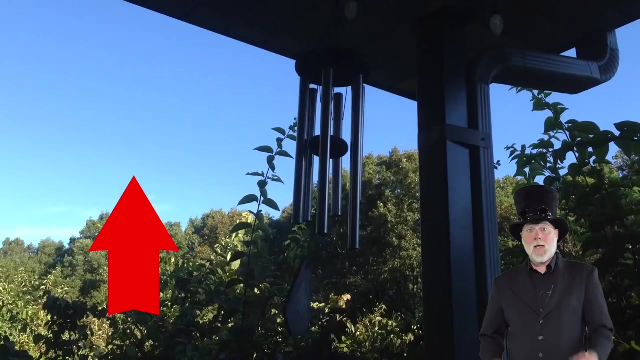 It's a cycle. The cool thing is, water is moving naturally through the water cycle And the energy in that movement can be harnessed by humans. as renewable power. Wind energy comes from solar heating of the Earth, from the sun. The heated air rises and the cooler air moves. 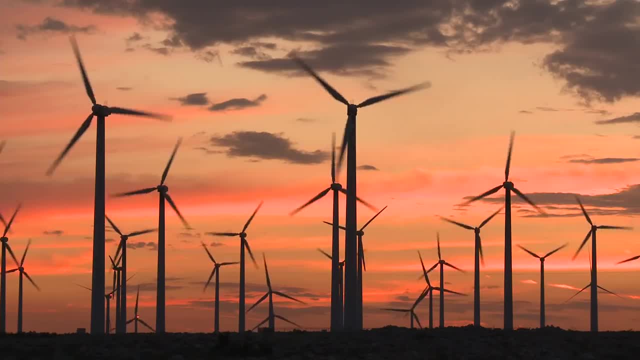 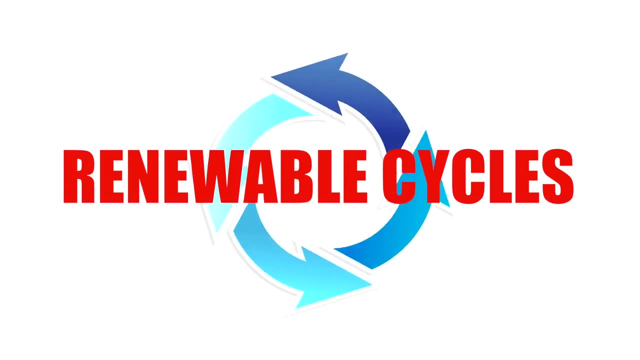 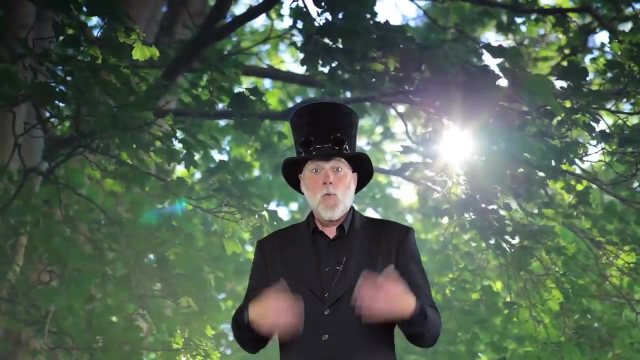 in to replace it, Ta-da. We have wind. The wind energy can be converted to energy that humans can also use. There are cycles all throughout nature. The oxygen we humans consume to live is replenished by natural cycles. We exhale CO2, carbon dioxide, which is absorbed by plants. 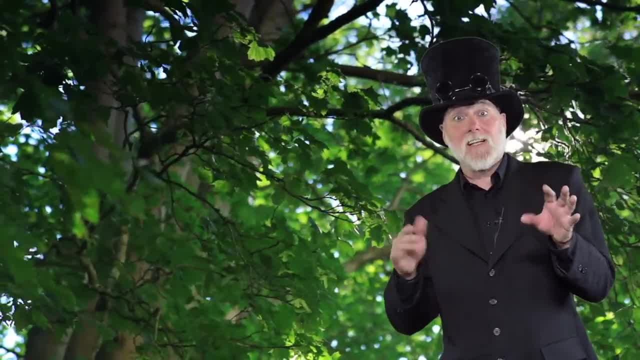 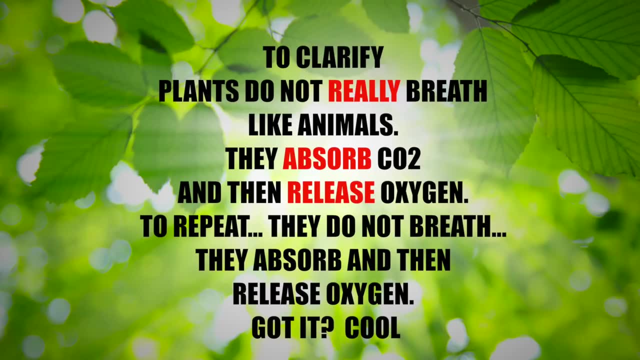 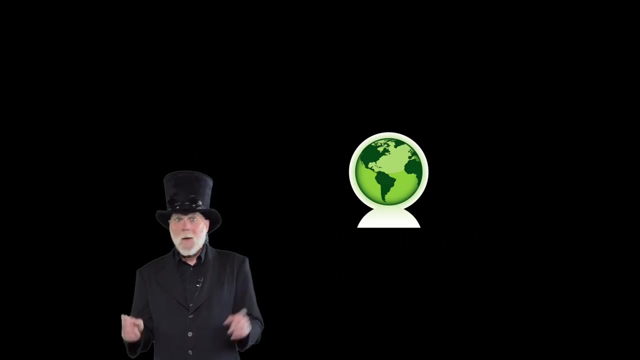 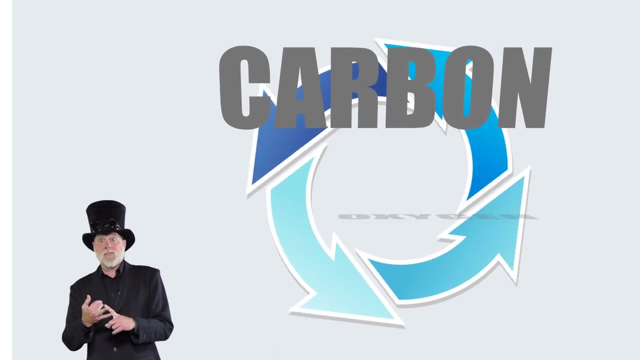 And then, in combination with sunlight, in a process that we call photosynthesis, they exhale oxygen, Oxygen that we can breathe. It's replenished by nature. There are lots of cycles in nature: The Krebs or nitrogen cycle, The carbon cycle. 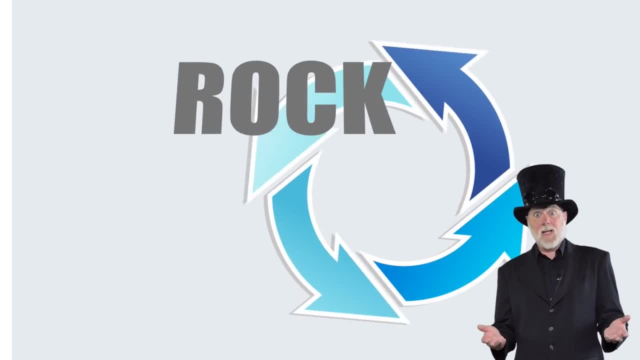 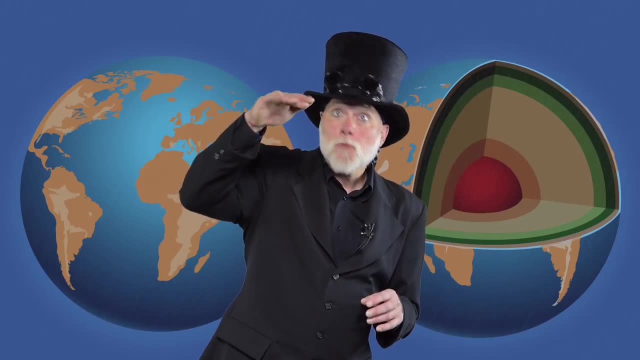 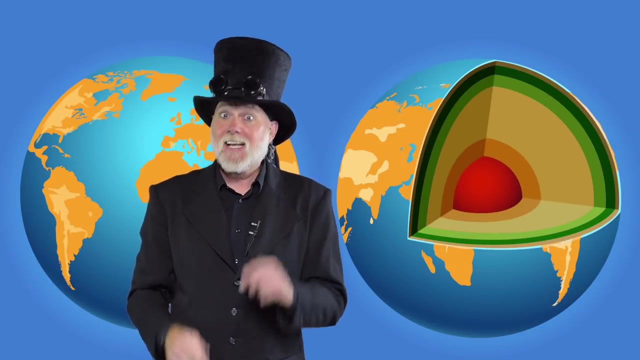 The oxygen cycle, The water cycle. There is also a rock cycle. There are even cycles within the Earth, like geothermal energy. The water starts as rainwater that has fallen to the surface of the Earth Percolates down to a magmatic- not magnetic- heat source in the Earth. 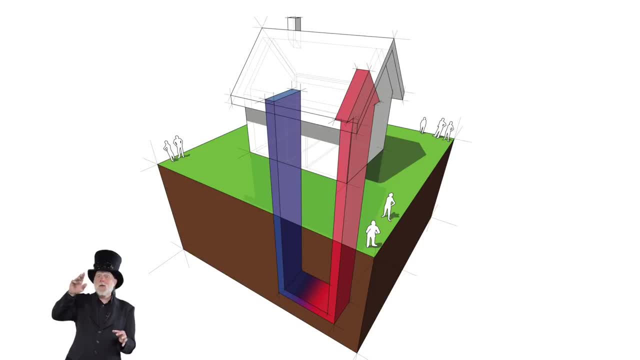 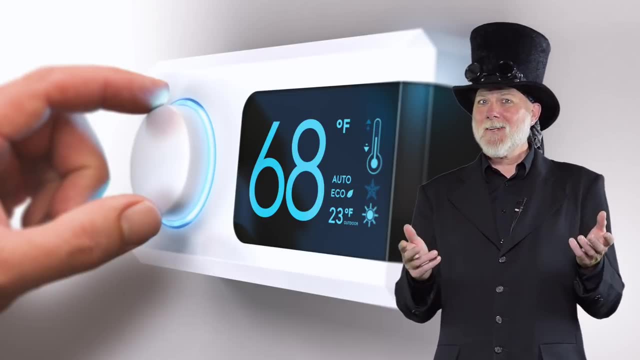 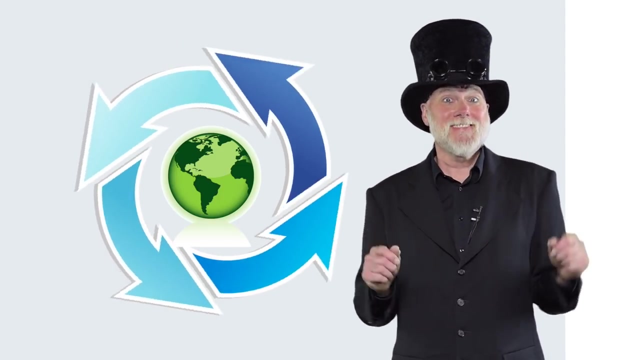 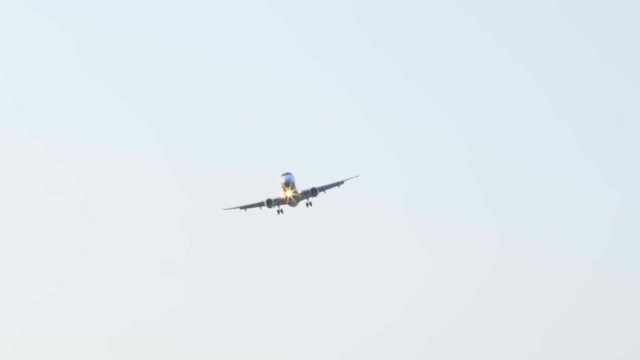 That heated or hot water now rises back to the surface because it's lighter, That hot water can be used as energy by humans and the cycle starts all over again. This cycle is continuously replenished by nature. Fossil fuels, natural gas, coal oil are valuable and powerful sources of energy for humans. 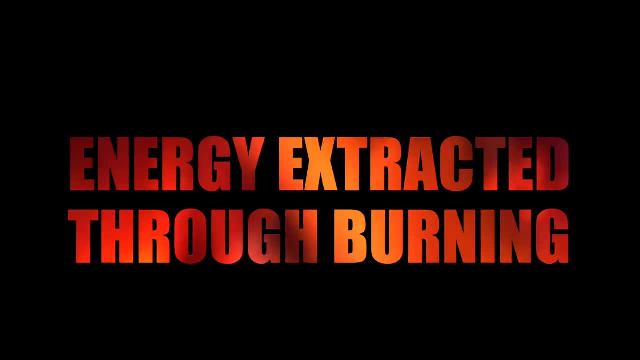 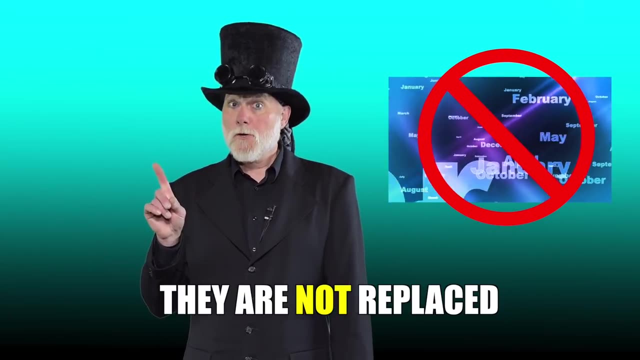 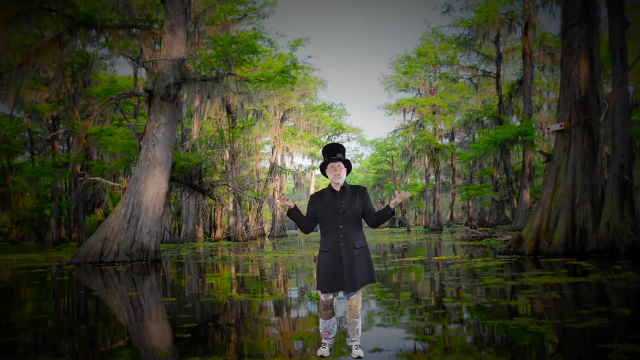 We make use of them by extracting the energy they contain by burning them. They are, however, non-renewable on a human time scale. When used, they are not replaced. Coal is a fossil fuel. It began as plants in a swamp a very, very long time ago. 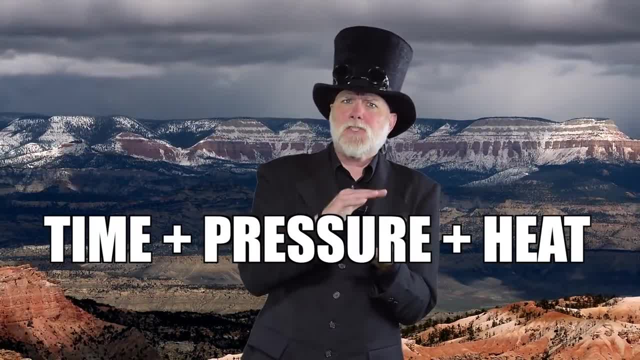 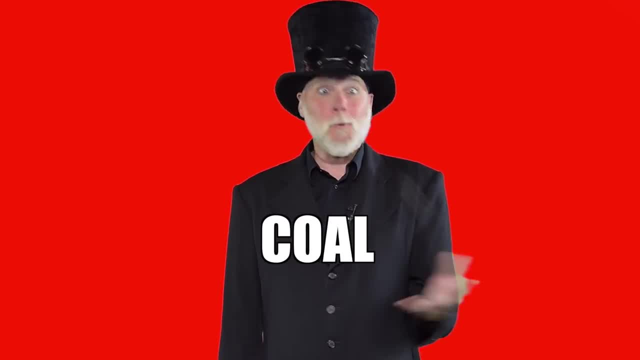 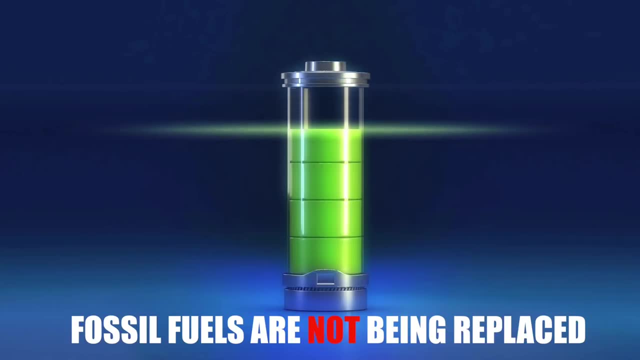 After the plants died, thousands of years of pressure from sediments pressing down, combined with heat, changed those plants into coal. Fossil fuels are extremely important. They are extremely useful to humans, but they're not being replaced as quickly as they are being depleted. 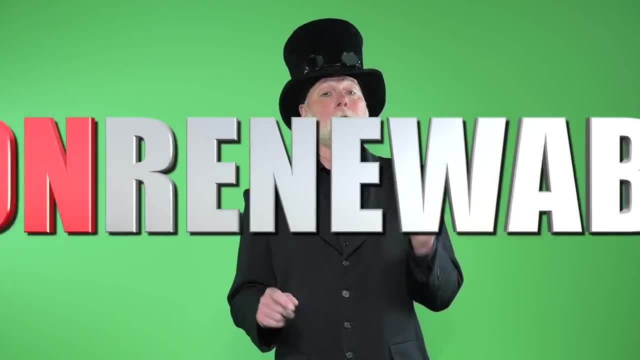 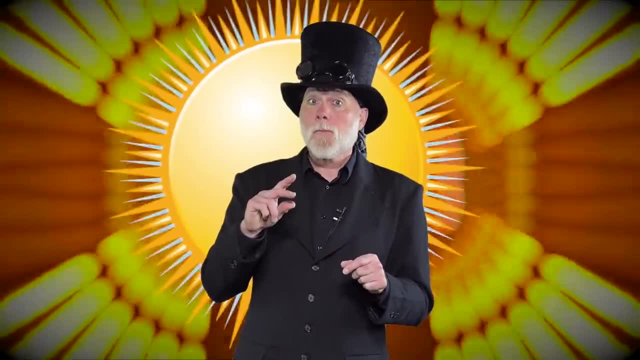 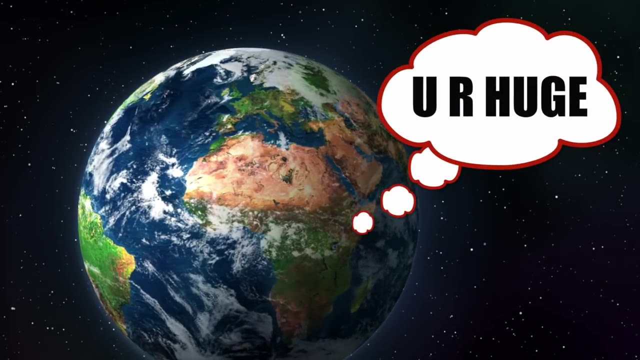 So eventually they'll be used up. They are non-renewable. The sun is an interesting case in the renewable versus non-renewable conversation because the sun is really huge And technically its energy is non-renewable- It's not being replaced. 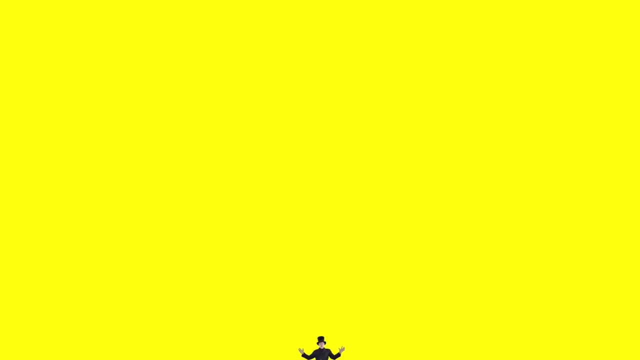 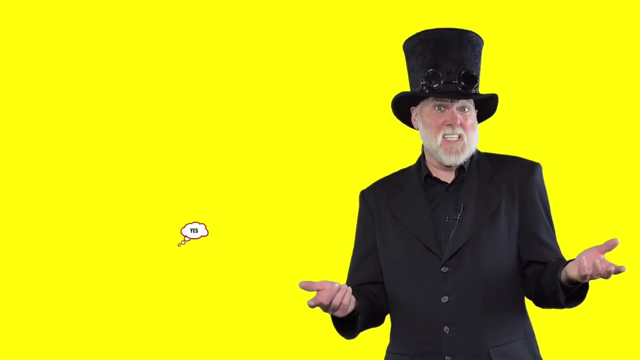 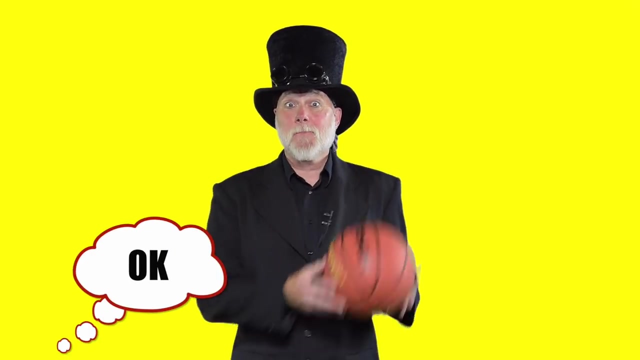 Thank you, But the sun is soooo huge, The use of the sun's energy by humans will not use it up. That's kind of hard to believe, isn't it, That something could be that huge. Imagine that the sun is the size of a basketball. 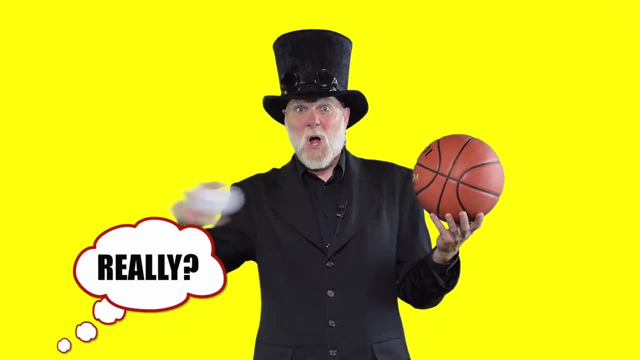 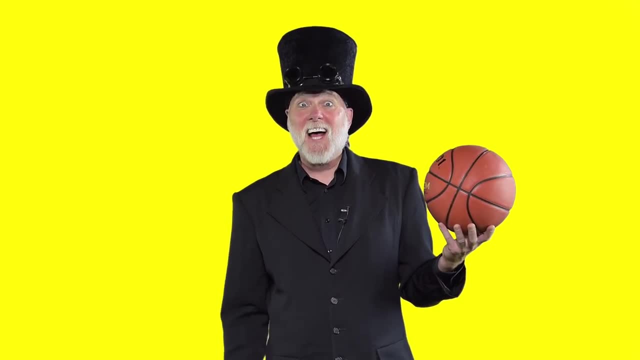 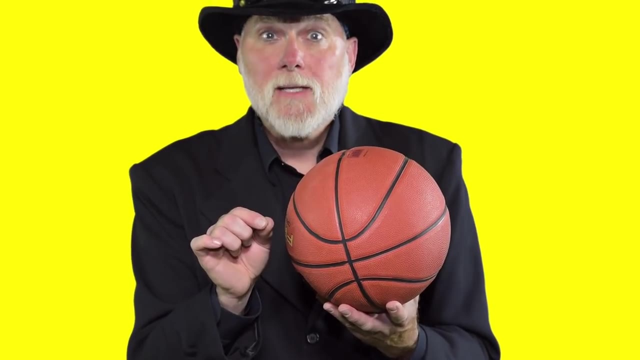 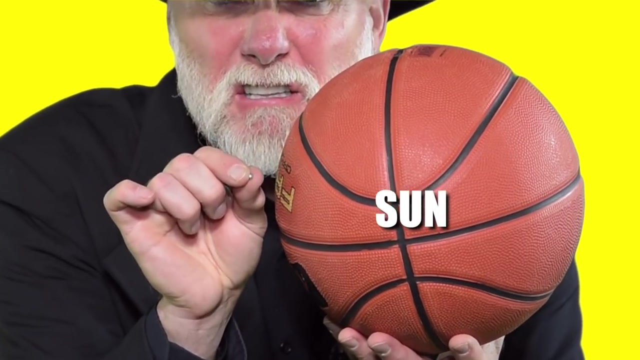 Then that would mean that the earth is the size of this wiffle ball. Nope, This eyeball- Nope, The earth would be the size of this teeny ball. That's right. If the sun were the size of this basketball, the earth would be the size of this itty bitty. 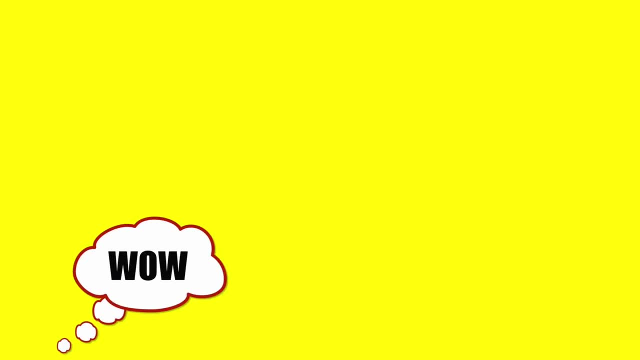 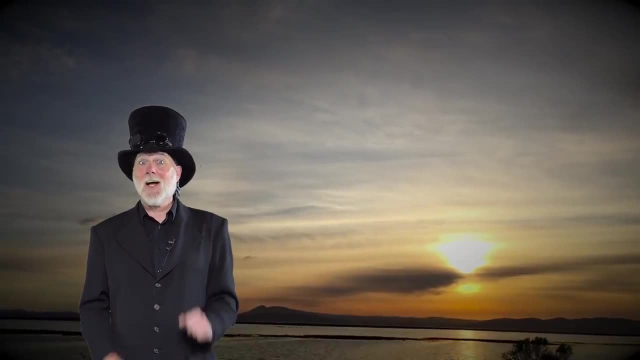 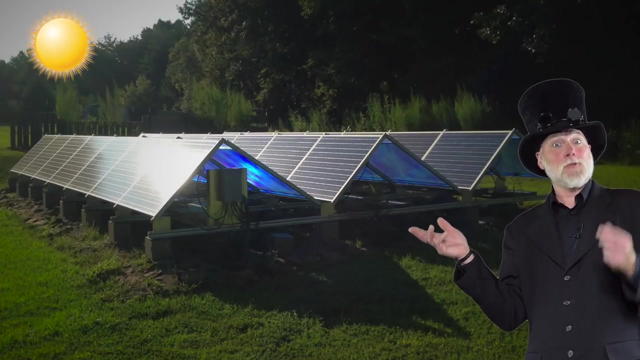 little bb. That means there's a lot of solar energy available to us earthlings from the sun A lot. I even have a 21-panel solar array in my front yard To capture the sun's energy And to use it in my home and TV studio. 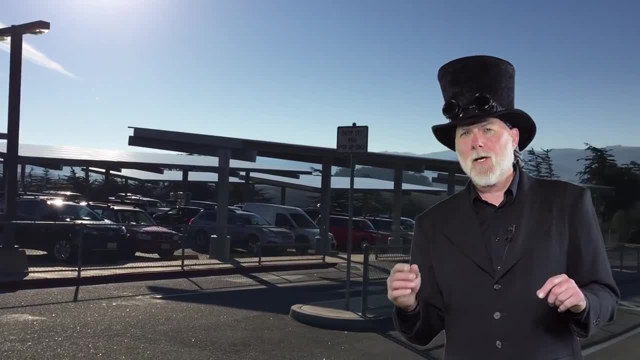 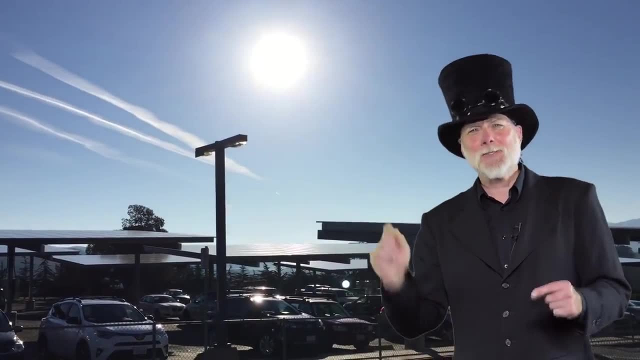 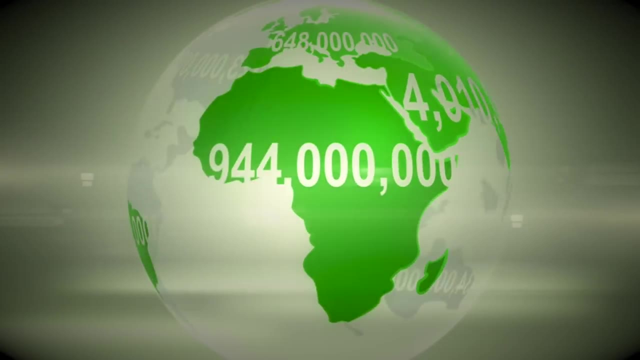 I once visited an elementary school in Southern California that had solar panels over its parking lot. It used that energy to power the elementary school. Cool right. These days there are lots and lots of humans. Energy is necessary for all human activities. 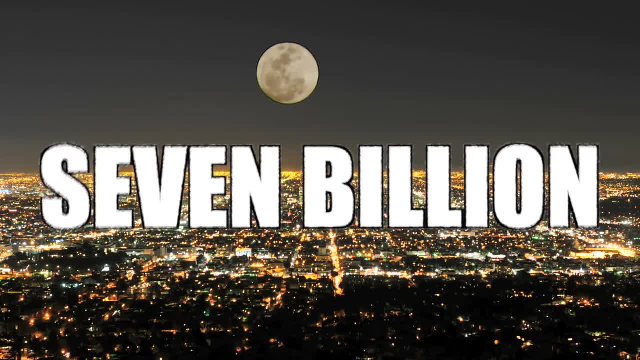 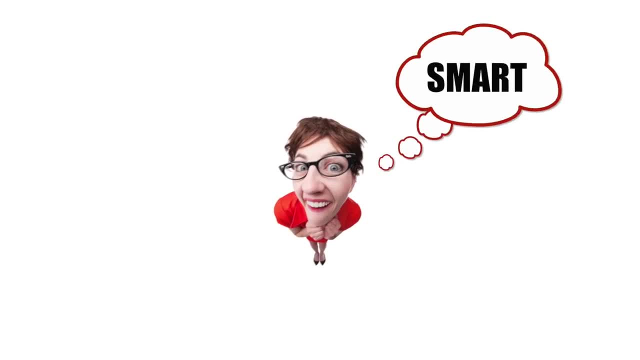 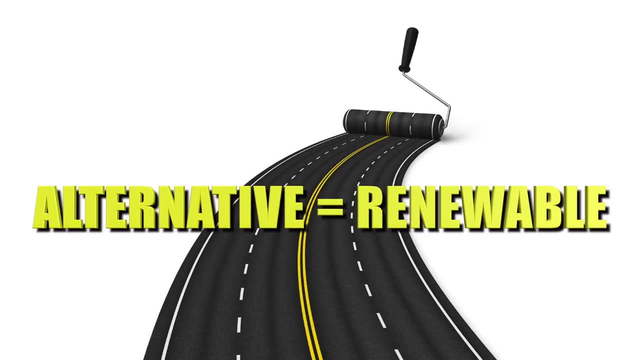 Right now, there are about 7 billion of us. That's the most in all of human history And the most in all of human history. Using nature's resources in very smart ways is really important. Alternative energy resources are considered renewable resources and rely on natural processes. 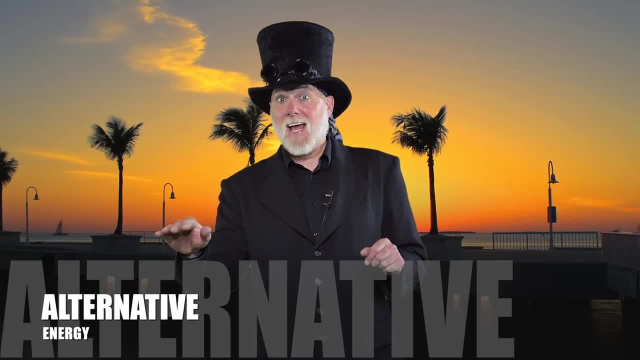 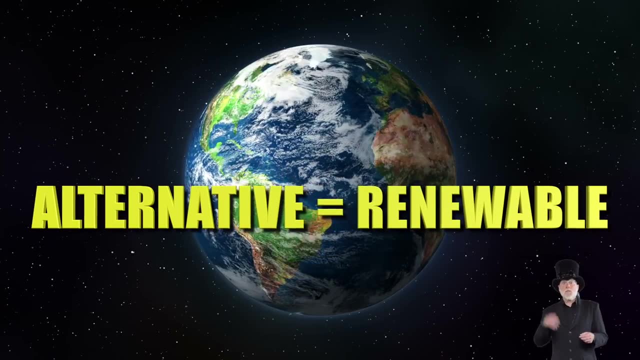 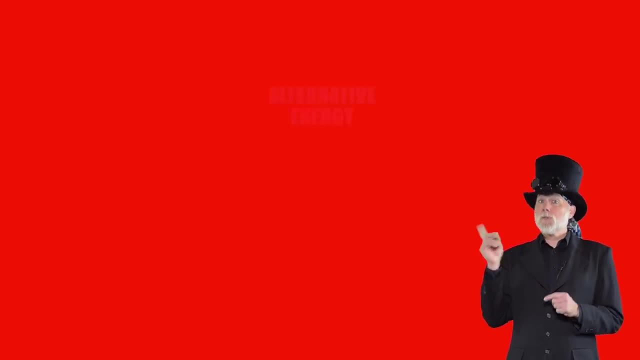 Flowing or moving water, sunlight hitting the surface of the planet, heat in the core of the planet, the movement of air, plants growing and dying are all part of the earth's natural systems. energy that humans can use. Alternative energy resources include sun, wind. 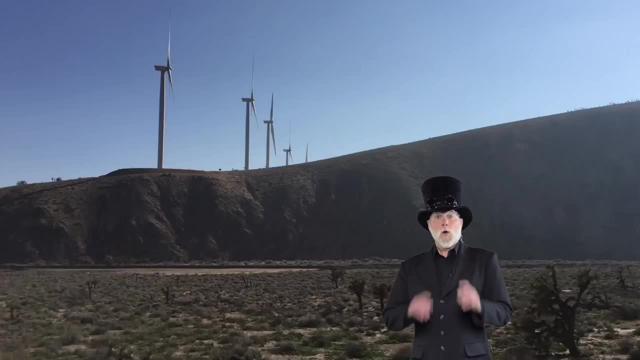 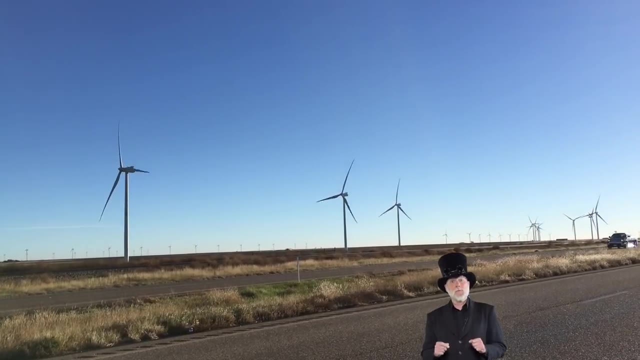 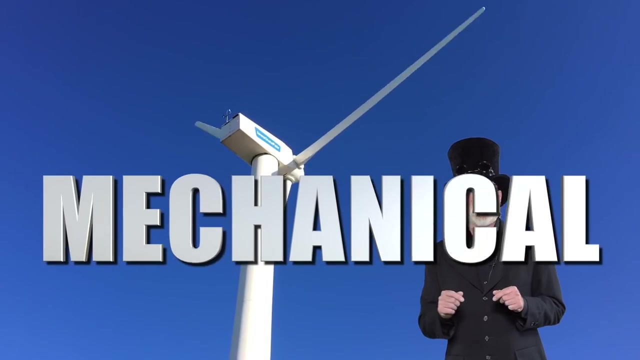 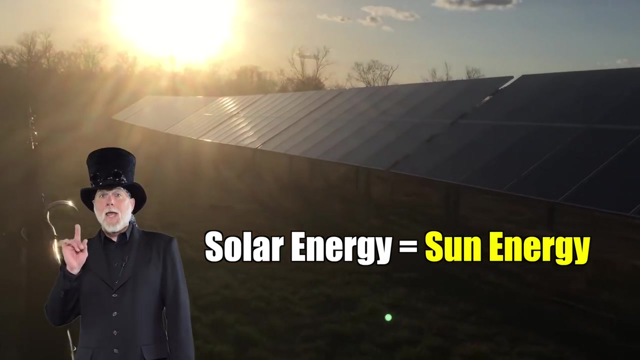 geothermal, biofuels or biomass. Wind energy comes from changing the power of moving air into a useful form that we can use. Wind can be captured by wind turbines that spin and produce mechanical energy, which is converted into electrical energy which we can use: Solar energy- Energy coming from the Sun. 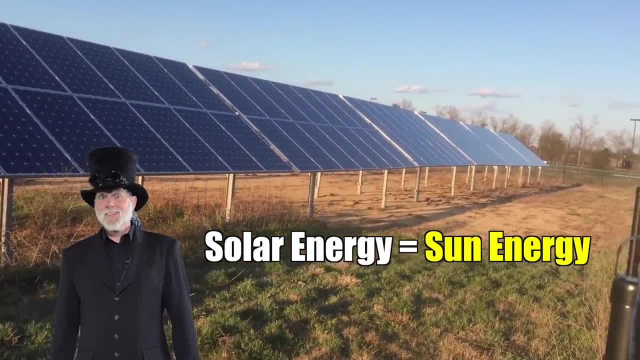 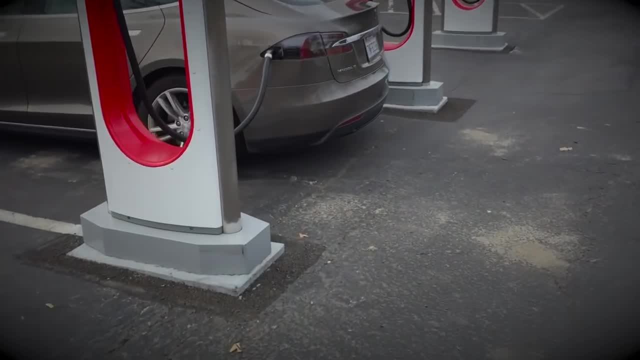 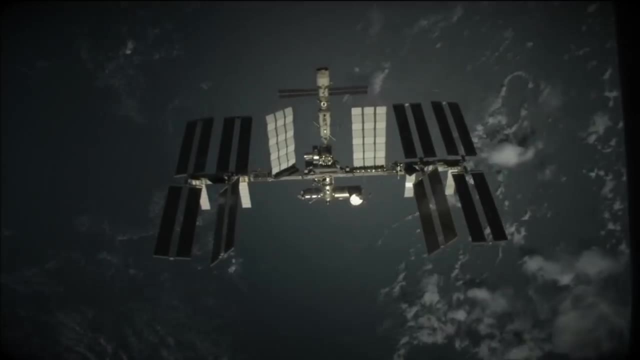 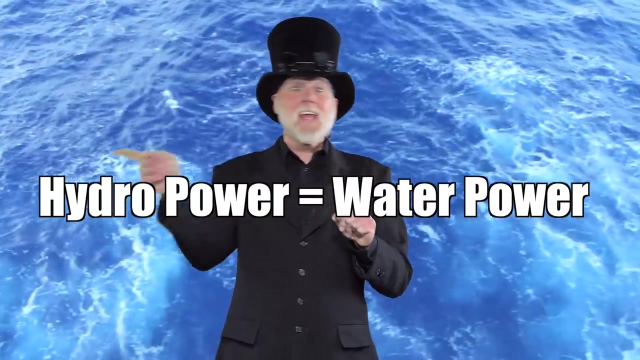 is converted to electricity that we can use. Sunlight hits a solar panel, The solar energy is converted to electric energy and we can use it- Hydro or water power. Hydropower is energy captured from moving water. Hydroelectric energy is created by a. 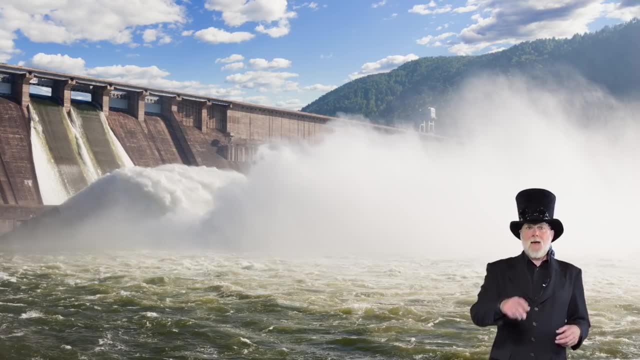 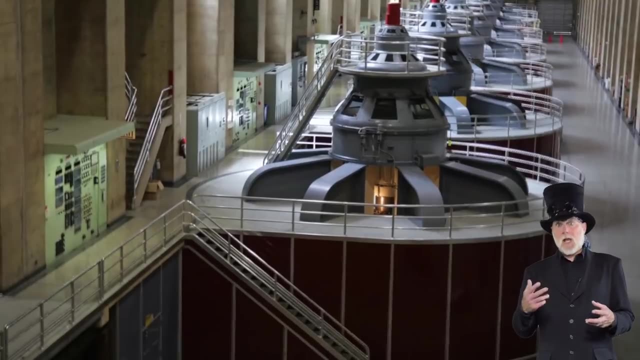 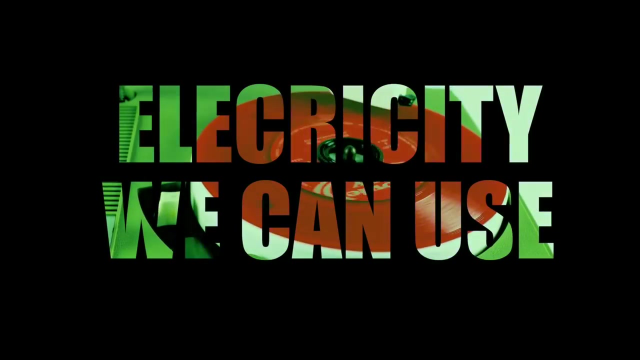 dam Falling water driven by gravity, a natural system turns a turbine, which creates mechanical energy. A hydroelectric generator converts the energy into electricity that we can use. Tides on the oceans can also accomplish the same thing. Energy from the movement of water, of tides, can be. 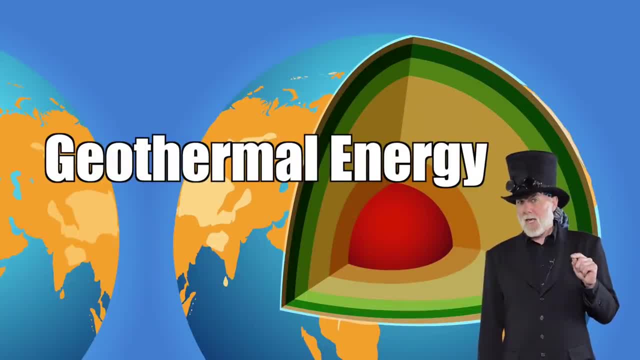 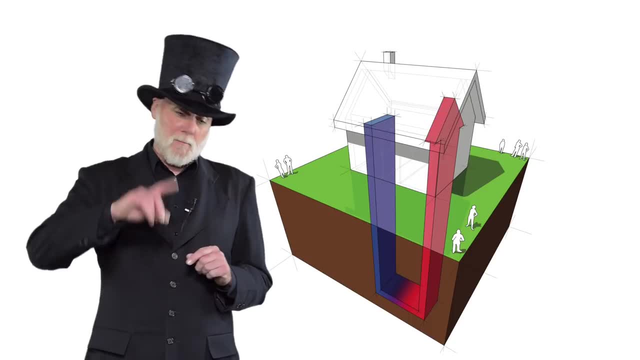 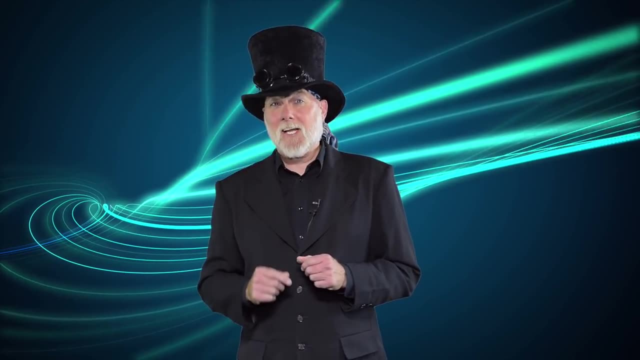 captured as energy by humans. Geothermal energy uses heat from inside the earth. Hot steam and water can be tapped by wells and brought from deep beneath the earth's surface. The steam can be used to spin turbines to generate electricity, or the energy from the heat can be extracted directly from the pipes for 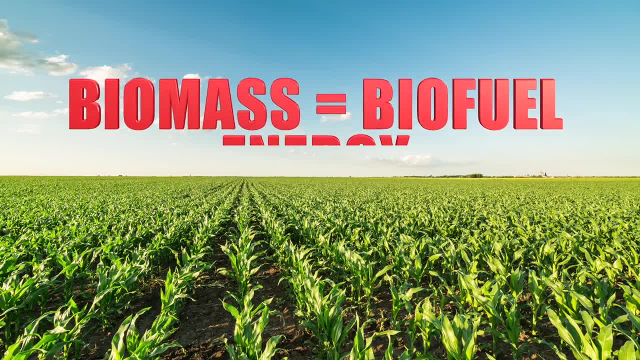 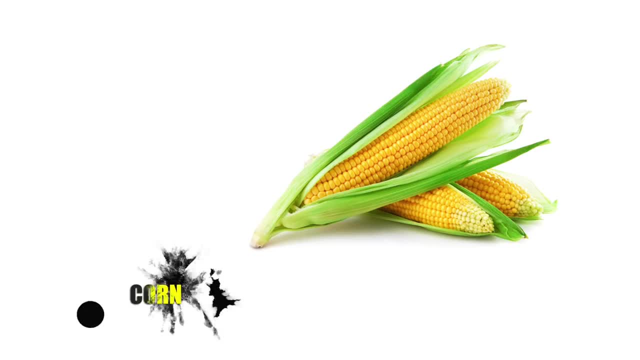 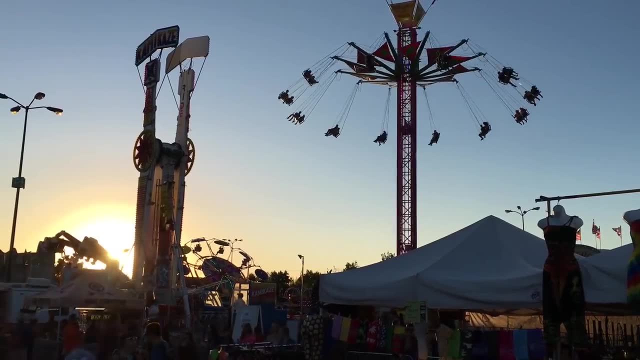 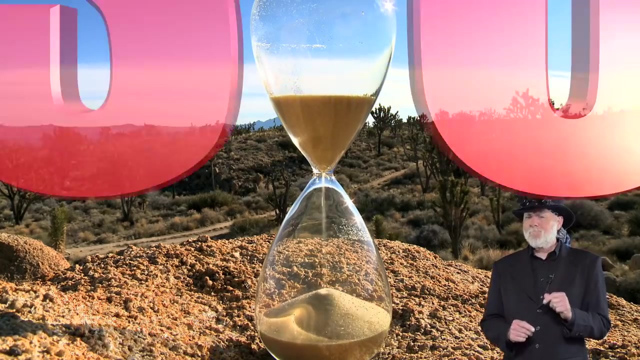 humans to use as energy. Biomass or biofuel. energy is fuel made from plant or animal waste. Energy from the sun is stored in plants. That energy is then converted into a solid liquid or gas that can provide energy for human use. Non-renewable resources exist in a fixed amount, so once used up, it's going to. 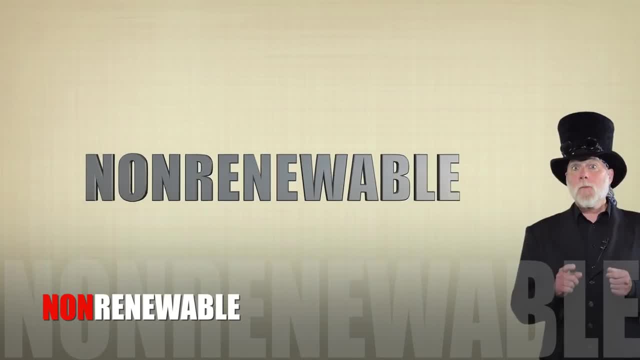 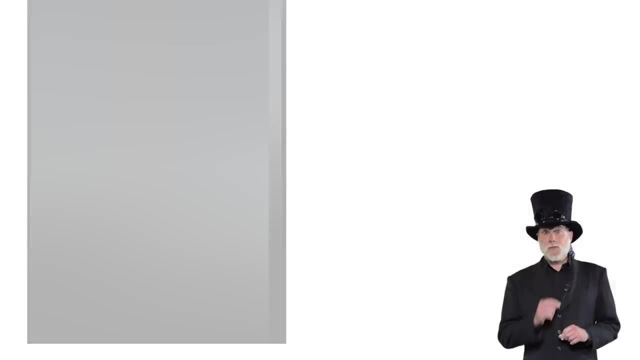 take millions of years to make more Non-renewable resources. energy and gas will be converted into a source of energy. Non-renewable resources are include coal, natural gas, oil and nuclear energy. Fossil fuels are pretty amazing. 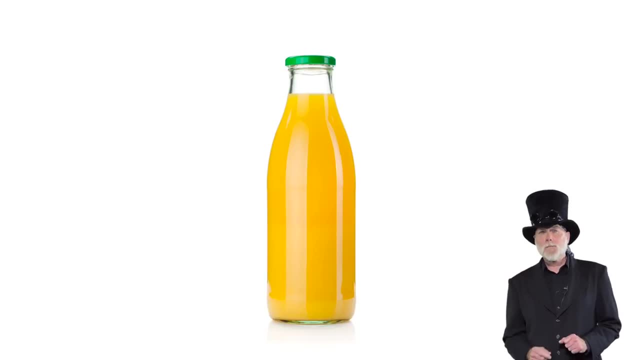 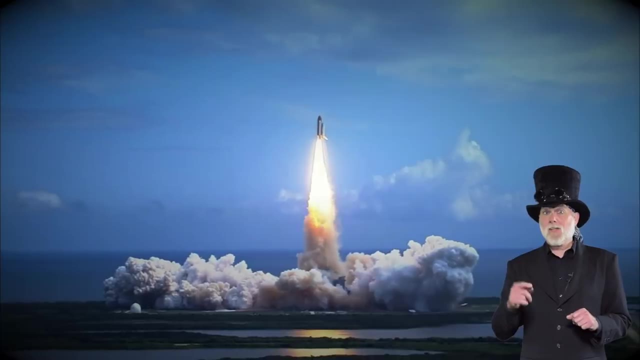 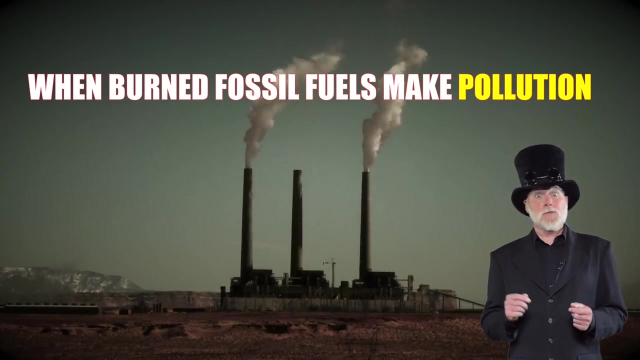 They've allowed humans to grow more food than ever before, design and build space-age homes that can control light and temperature, and even travel outside our biosphere to the moon and beyond. Unfortunately, when burned fossil fuels create hydrocarbon pollution that harms the planet.